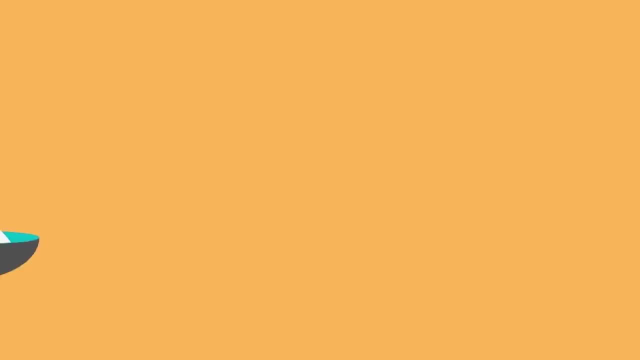 quickly reactants decrease is a reaction between marble chips, calcium carbonate and hydrochloric acid. This reaction can be represented by the following equation, made up by the reactants calcium carbonate and hydrochloric acid, resulting in the products calcium chloride and water and carbon dioxide. As the reaction proceeds, the reactants lose mass because 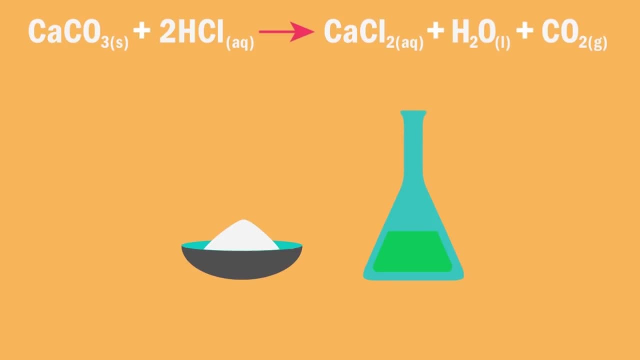 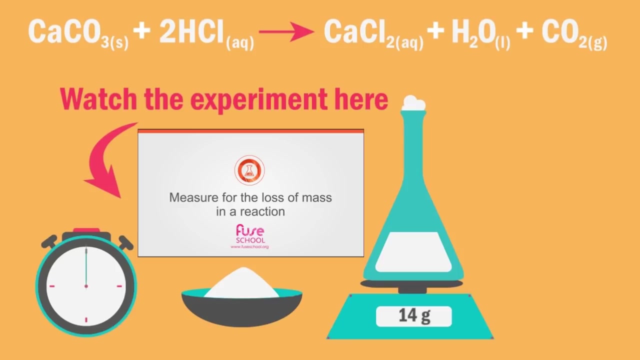 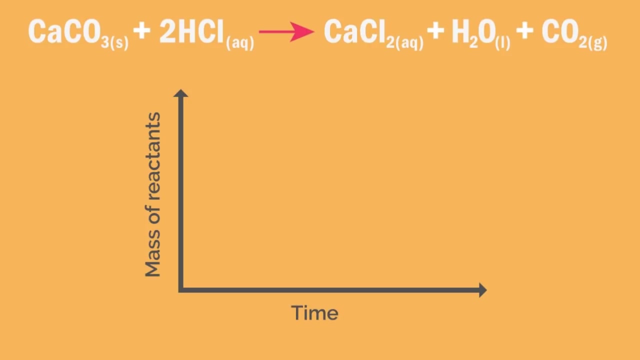 carbon dioxide gas is given off. We can measure the decrease in mass of reactants by using this type of apparatus. Based on our measurements, we plot a graph of mass of reactants against time which looks like this: The rate of reaction at point A is given by the gradient at A, which is y over x, And the 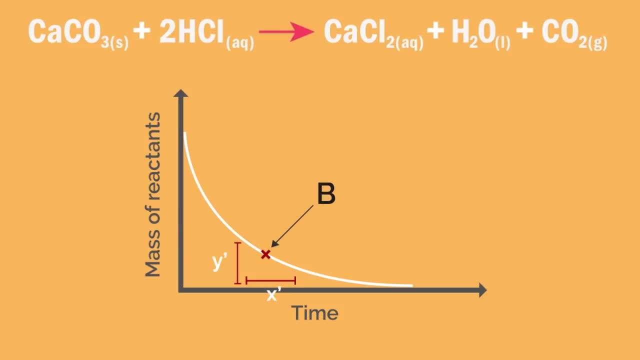 rate of reaction at point B is given by the gradient at point B, which is y dash over x dash. What do you think is happening to the rate of reaction at point B? Let's take a look at the reaction as it proceeds. Pause the video here. Give it a think. 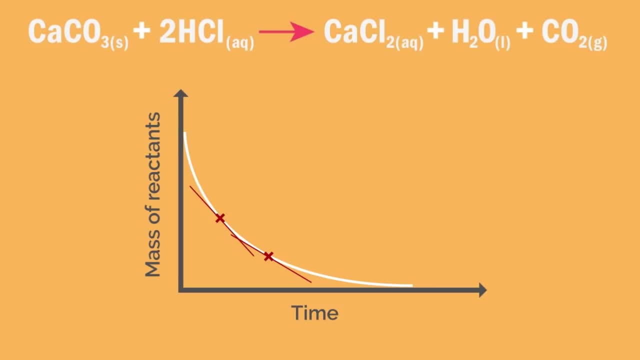 The answer is that the rate of reaction slows down, In other words, the rate decreases. Did you get it right? Do you remember? there's another method we mentioned earlier. Consider the same reaction. Instead of measuring the loss of mass of the reactant we can measure. 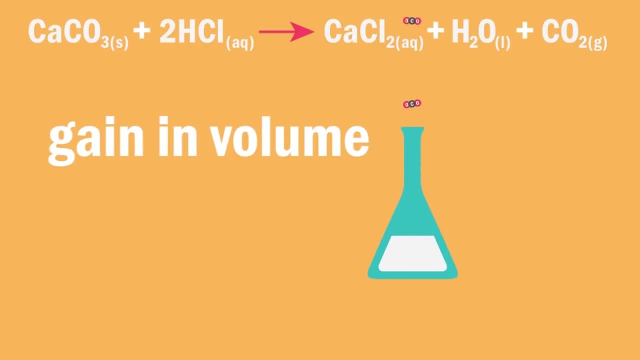 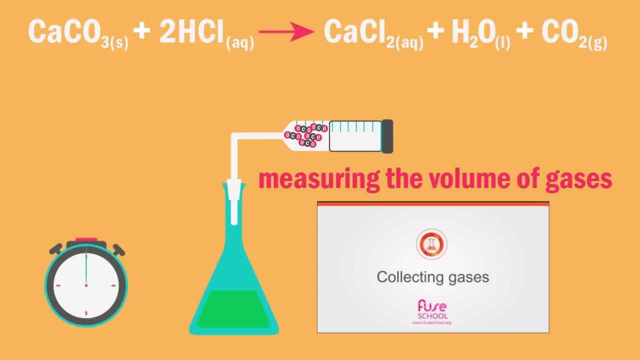 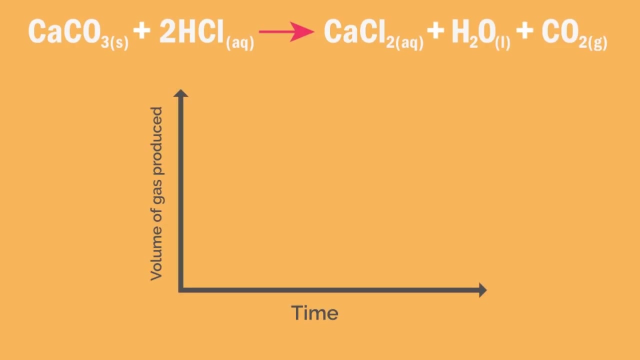 the gain in volume of the product Carbon dioxide Using an apparatus like this. You can watch our video on measuring the volume of gases here. This time we plot a graph of volume of gas produced against time. The graph looks like this: 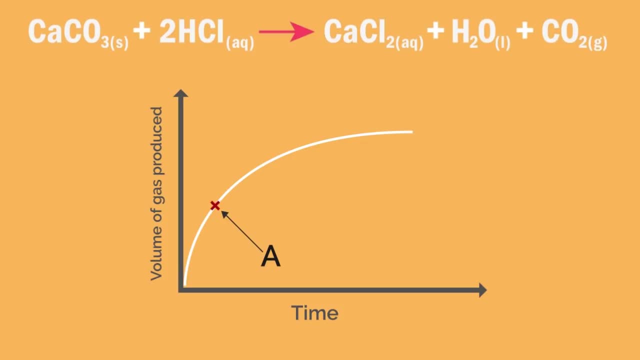 As before, the rate of reaction at point A is given by the gradient at A, which is y over x, And the rate of reaction at point B is given by the gradient at point B, which is y dash over x dash. What do you think happens to the rate of reaction as it proceeds Again? pause the video here.